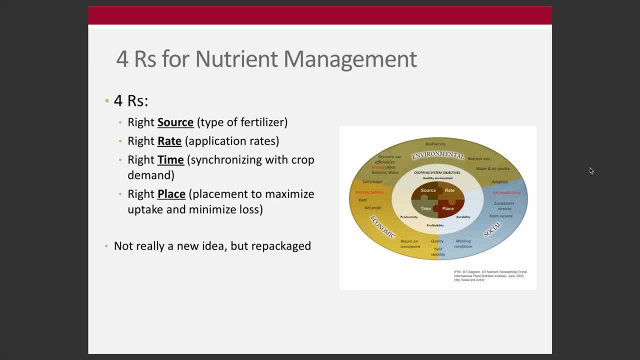 What is the fertilizer that you're using, What is that source? And then the rate is actually how much you're applying. Timing deals with when it's applied. Is it applied in the fall at planting? mid-season Placement is how it's placed. Is it broadcast? Is it banded, Et cetera, et cetera. 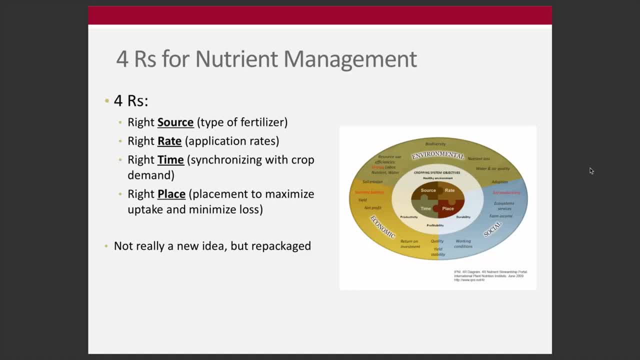 So there used to be an organization, IPNI And International Plant Nutrition Institute. this was a fertilizer industry kind of scientific branch of the fertilizer industry. They did a lot of good things, made a lot of materials. You're going to run into some of their materials in the course of your career. 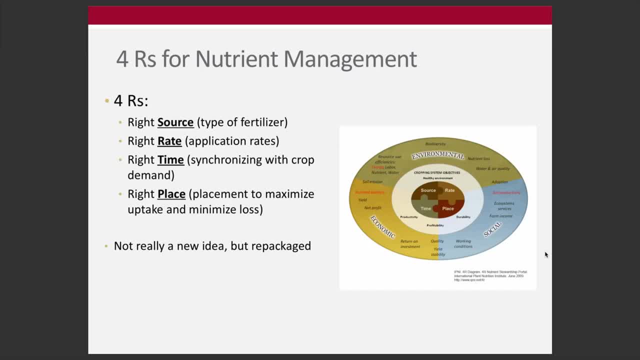 Unfortunately, they have lost funding and they have essentially been disbanded, and so a lot of that responsibility has been taken up by the Fertilizer Institute. It's really unclear what that's going to look like, but you know it's a bit of a digression, but IPNI is widely credited with this concept and this packaging of the 4-R, so just something to be aware of, okay. 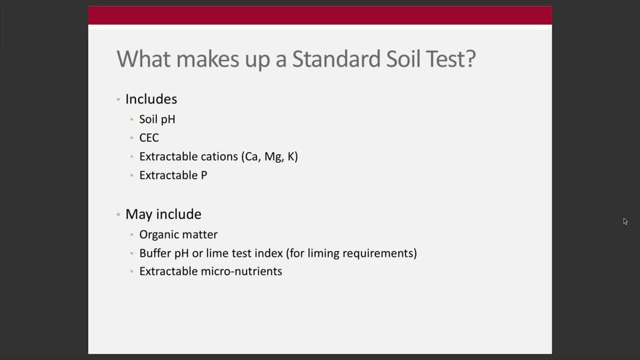 And we've talked about what makes up a standard soil test a little bit, but let's kind of dive into this again. And so when you pull a soil sample and you contact a commercial lab and say I need, you know, a soil analysis done and this is you know. of course there's lots of different measurements in soil science. 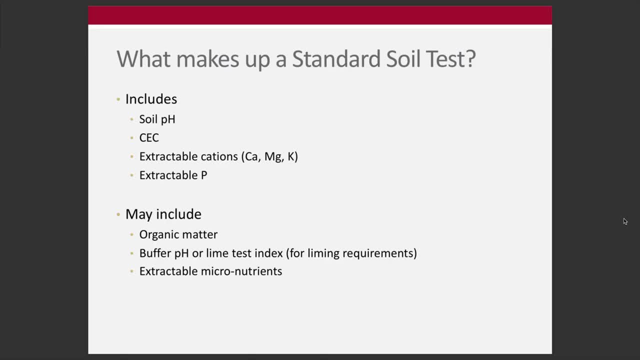 but what I'm talking about are commercial soil testing labs. okay, They're often going to have packages. We've got an S1, an S2, or an S3, or we've got a you know soil one or like whatever, but quote-unquote, a standard package that they offer. 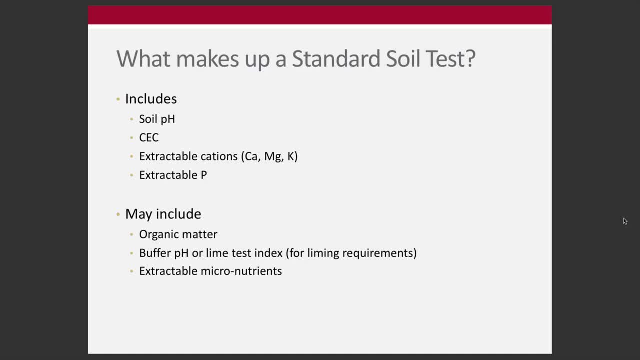 and that nearly always includes soil, Soil pH, a CEC, that's cation exchange capacity, of course extractable cations of calcium, magnesium, potassium and then extractable phosphorus. So almost every commercial lab is going to offer you that as kind of the fundamental baseline. 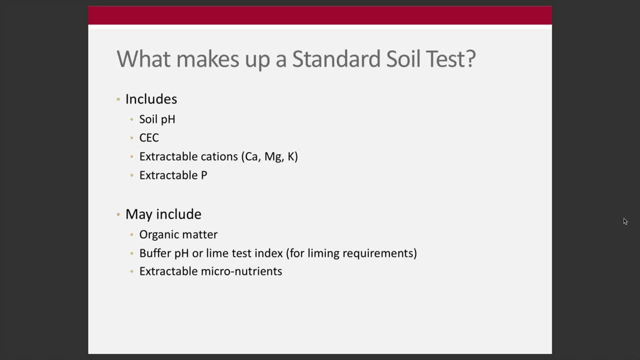 Their packages may also include things like organic matter percentage, a buffer pH, which we've already talked about, you know for that liming right, Right, Right- And then possibly extractable micronutrients, things like boron, zinc, manganese, et cetera, et cetera. 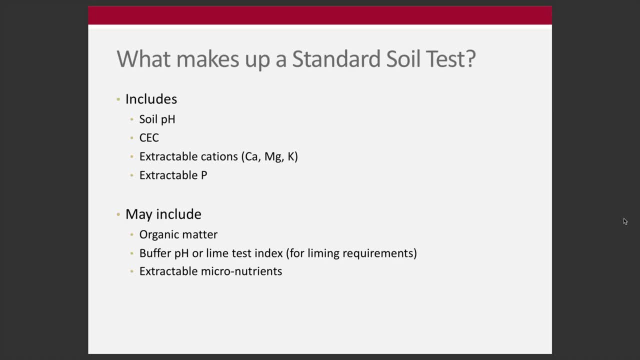 So that's really what's kind of the foundation, of the bread and butter for a lot of soil testing. Now, note we've already talked about this, but note that nitrogen- a measurement of nitrogen- typically isn't included, right? So soil nitrogen isn't directly measured many times. 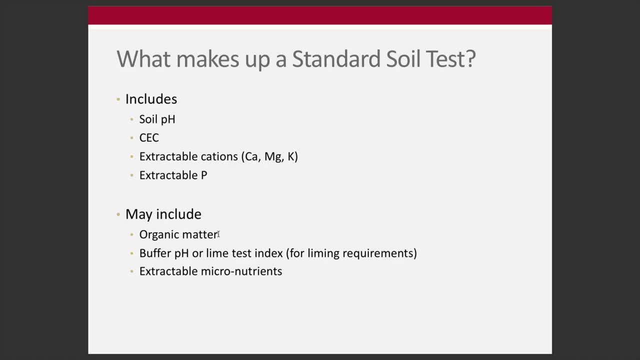 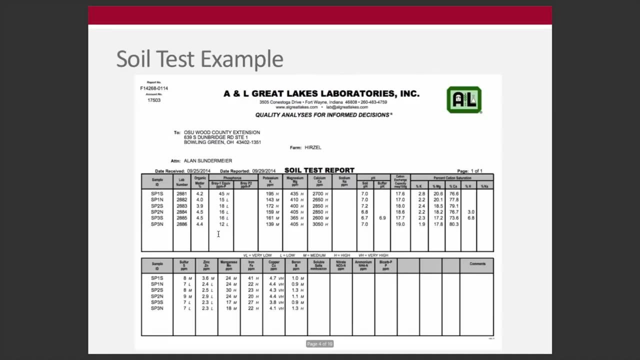 Some people say, oh, if you, If you get organic matter, you're going to have a sense of that, and that is true to some extent, but it's certainly not a really precise value. So soil tests, you know, depending on the lab that you send, we have a really rich infrastructure that is very easy to take for granted. 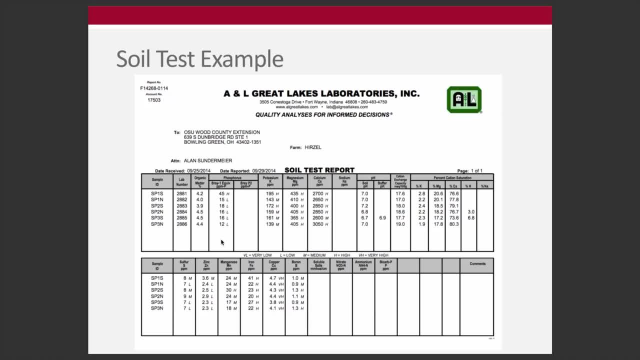 but there's been a lot of public investment over the last 60,, 70 years in figuring out how to take soil and find out its ability to supply nutrients to crops right, And so soil testing is a large industry and we are very lucky, very fortunate, to have a number of really good labs in the state and in the Midwest that can serve us and are happy to run soils for us. 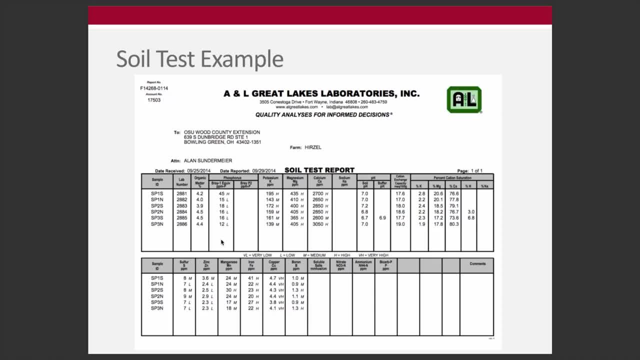 So if you've never submitted a soil sample or looked at a soil test report, they come in different shapes. They come in different shapes and sizes, but essentially here's a report with six soils in it or different sample IDs. The lab is usually going to give it some kind of internal number. 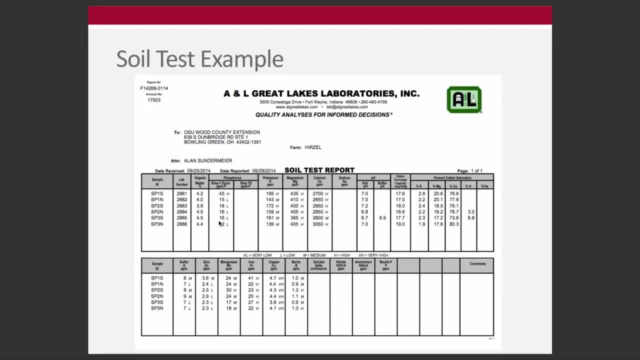 Here's organic matter, here's phosphorus and potassium, magnesium, pH, et cetera, et cetera. So we can go through some of these and we'll deal with a little bit more of this as we get into it. 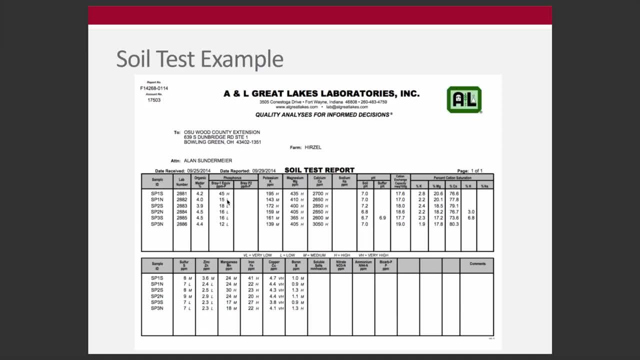 But what we can see? What we can see is that these values have an H, L, L, sometimes an M, H- and what does that mean? Or VH, so very high, high, medium, low or even a very low. 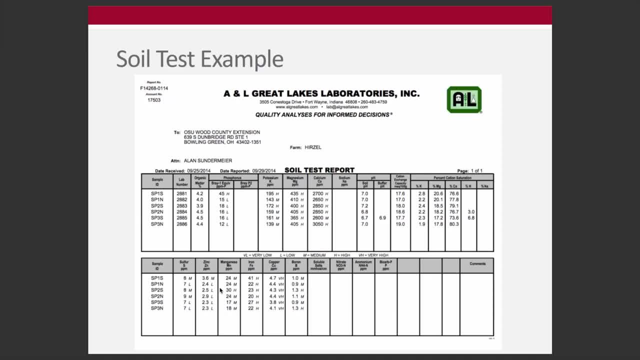 And so that's kind of a relative. It's a way for somebody that gets these results to understand: are these values good or are they bad, right? So? So an M would be- And again this is going to depend on the lab- but an M would be medium, that's kind of optimal or high, you know, depending on how they code these. 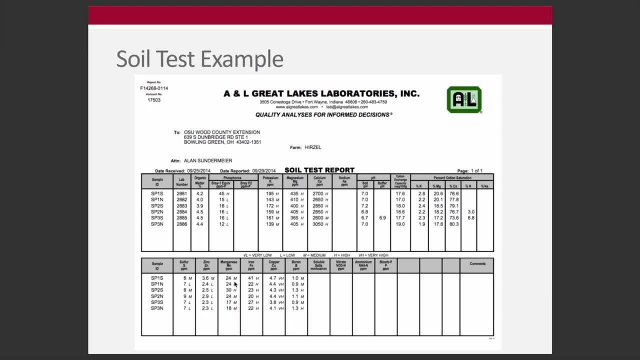 It differs by lab and depends on you know who's actually running that result. And you might say I'm growing potatoes and that might be very. Or I'm growing, You know I'm planting an apple orchard, And then if you tell the lab that these values might be coded very differently depending on the you know, on the nutrient needs of that crop. 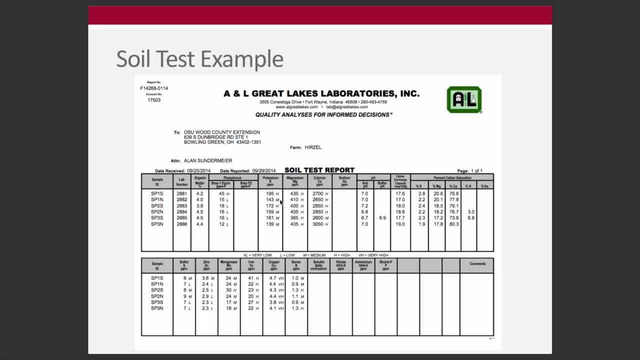 So it's important to understand, of course, that we can get a number, but knowing what that number means and how it relates to what we're trying to achieve can vary widely depending on the crop and on- you know, the interpretation of that. 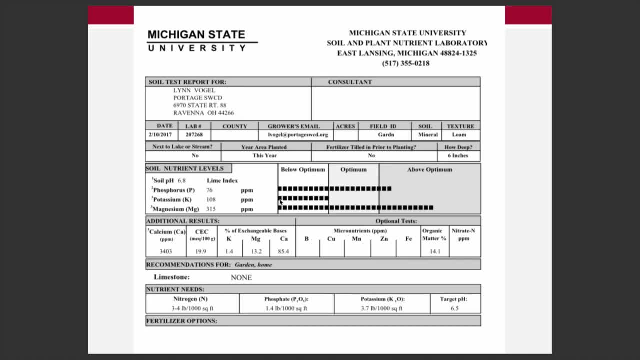 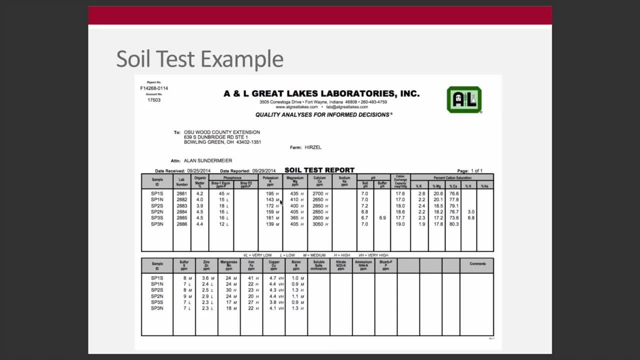 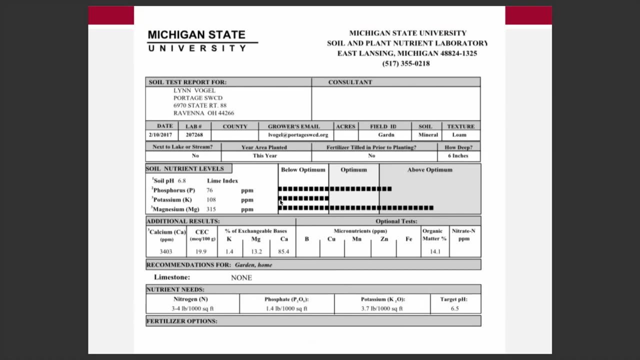 So you know, here's another, This is another. So this is ANL Labs out of Fort Wayne, Michigan, a very large lab that services a lot of northwest Ohio. Michigan State University has their own public lab. It's not particularly a large lab, but they, you know, they run. 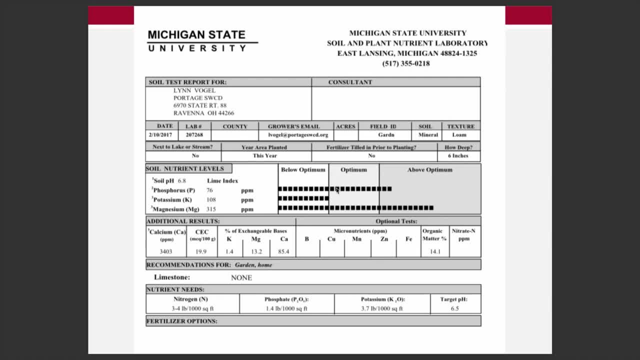 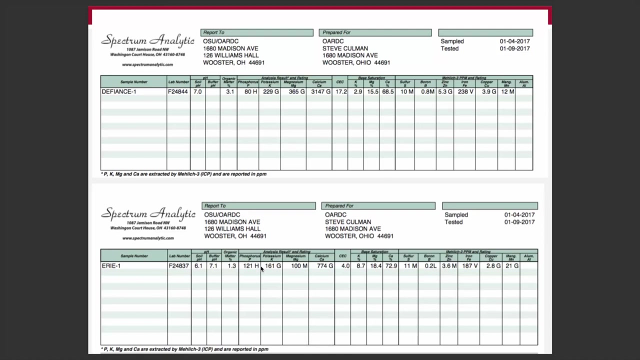 And they've got this: instead of a high, medium and very high or low, they've got low, optimum, optimum and above optimum. okay, So again, these are, And here you see, recommendations for a home garden And so if it was recommendations for, you know, a wheat field, it might be different and it would be different actually. okay. 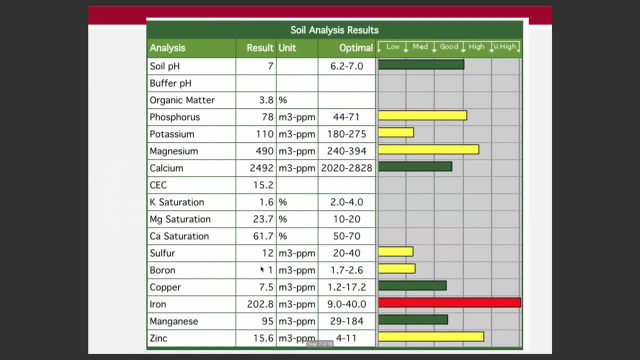 Just showing you some more examples of what this is. So you know this is a good example of you see the results. So here's kind of like the absolute number based on the different nutrients: Calcium, magnesium, potassium saturation. We talked about this already, right with the CEC section. 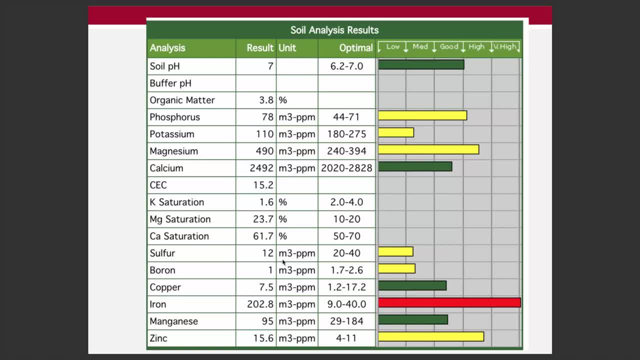 Here's the unit of measurement: either a percent or an M3, a malic-3 part per million. And then here is. So this is. These two columns are really like the values that you get, that are absolute in some ways. 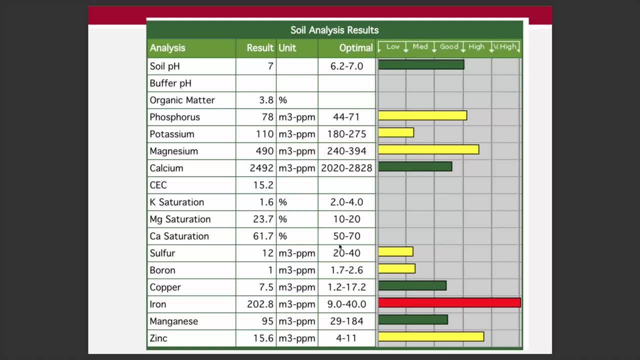 But then when we put this optimum column- And that's basically telling you what your soil test values should be, You can see, for organic matter there is no optimum because it depends on soil type. For pH we say 6. They're saying 6.2 to 7.. 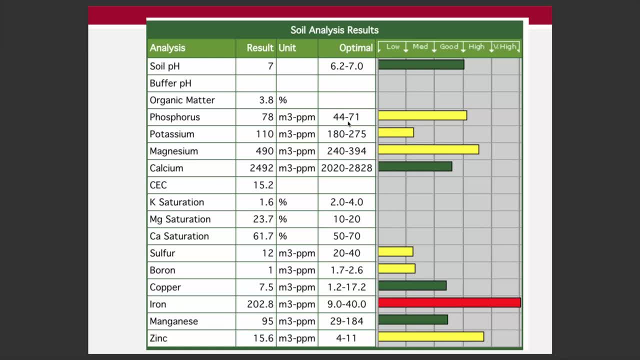 For phosphorus 44 to 71,, et cetera, et cetera. So part of this, what we need to understand is we can generate soil values But when we go to interpret them, if they're high, if they're good, if they're optimal, if they're too low. 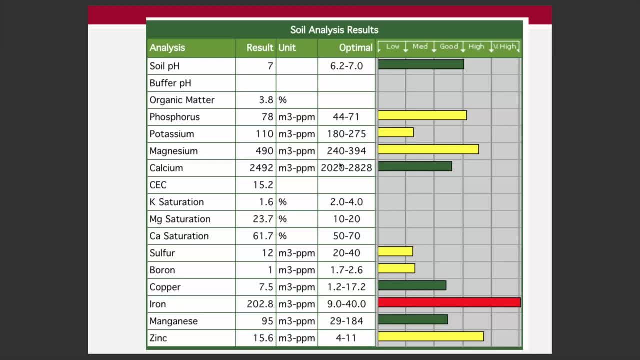 that's like a whole other step of interpretation, right? So again, where do these numbers come from? Where do these optimal ranges come from? How are they developed? Why is this green and this one's red and this one's yellow, et cetera, et cetera? 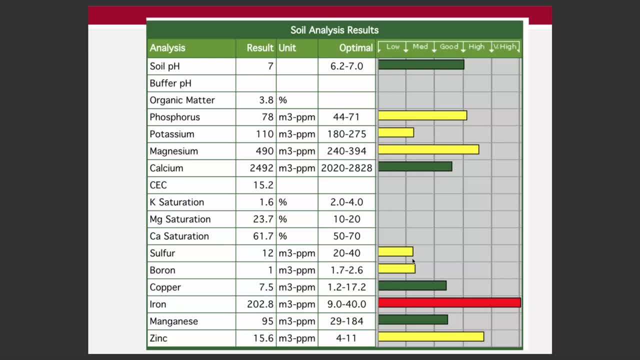 So we're not going to get into all this, But it's just important to recognize that. you know a value of 12 part per million sulfur. malic-3 sulfur might be optimal for or below optimal for one crop, but it might be above optimal- or you know whatever- for another one. 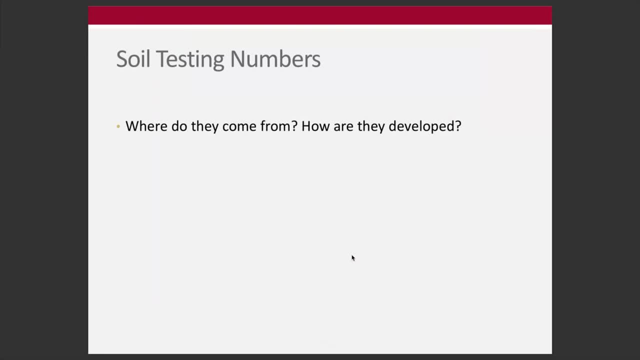 So where do they come from? Where are they developed? How do we actually get soil test numbers and provide interpretation for that? Okay, So there's a model, There's a mantra in soil fertility, and it's this idea of correlation, calibration recommendation. 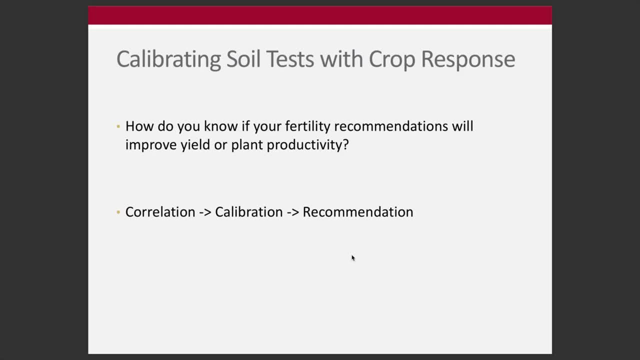 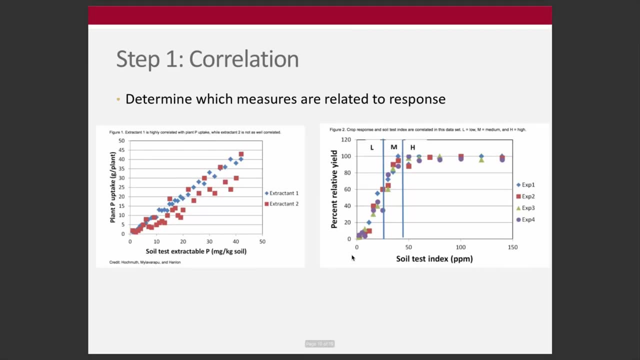 So these are three steps that occur in order of actually developing a fertilizer recommendation. okay, So again, correlation, calibration, recommendation. So let's talk about these. So the first one's correlation, which is determining which measurements are related to crop response. okay, 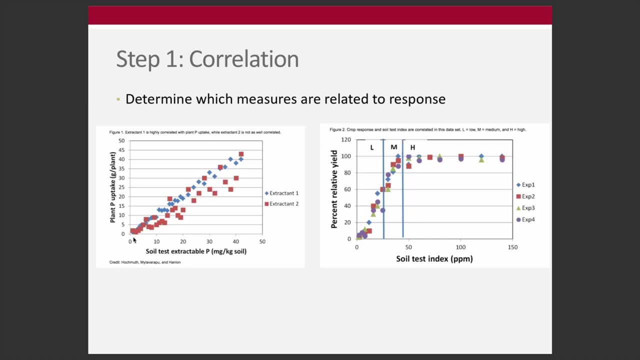 So here we've got something like plant uptake and soil test, extractable P. So we can see that as soil test P increases, maybe our plant uptake increases. But if we look at these two different extractants, there's a lot more variability with extractant two than with extractant one. 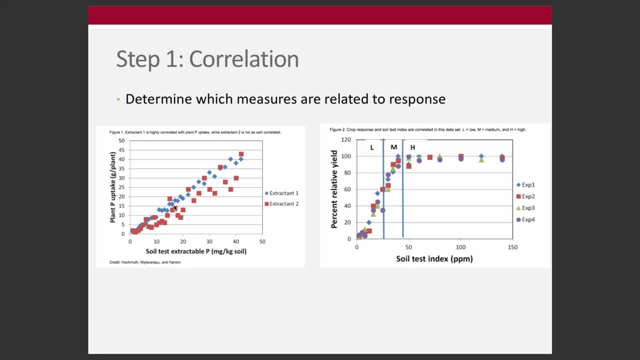 So maybe you know we do this work and we say: oh well, extractant one actually is performing better here, okay, And then we can think of taking some index of availability. So again, here's the soil test index. 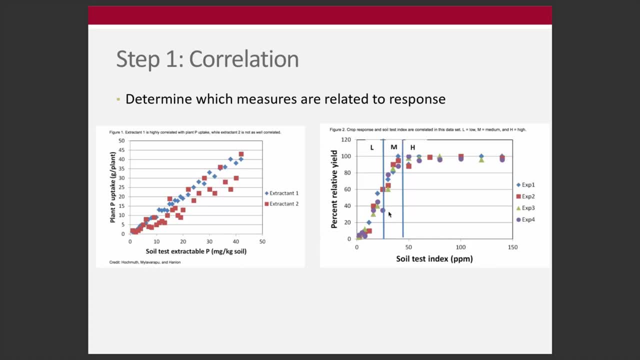 Maybe it's extractable phosphorus, And then we can see over time. maybe we run, you know, some various experiments here, one through four, and we see maybe this is like in a greenhouse or whatever, And we can see that it's somewhere above 50. 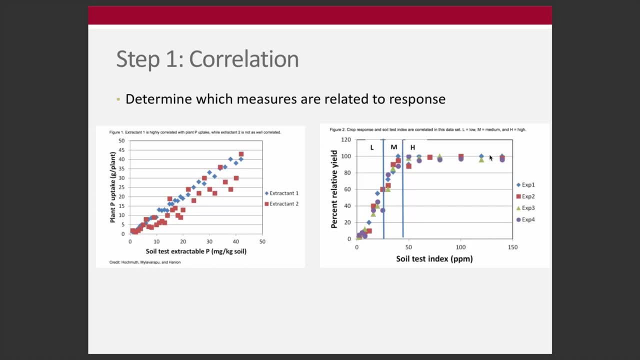 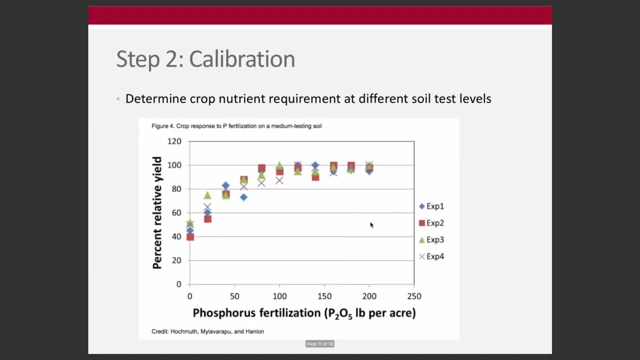 that no matter how much phosphorus we apply, we don't get any response. But when it goes below- maybe 50 or even 30, we start to see differences. that happen okay. So this helps kind of us actually correlate what things are. 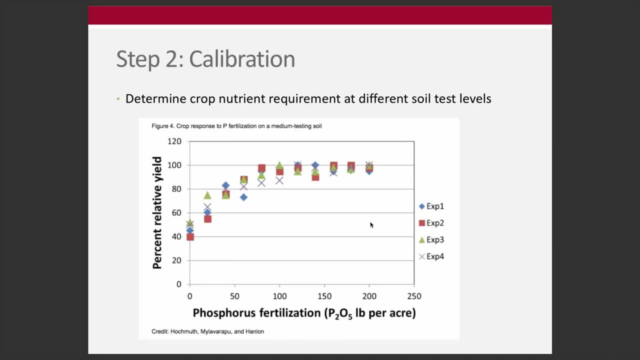 So the second step which can blend, of course the correlation and calibration work can blend together. but calibration is the second step And here we're actually trying to determine the crop nutrient requirement at different soil test levels. So we have imagine we have different soil tests. 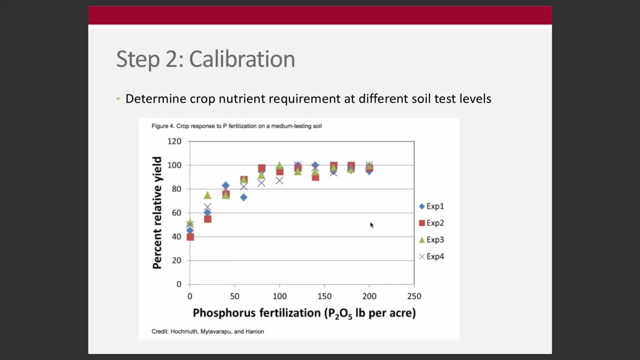 and we fertilize at multiple different rates. okay, We do this across a bunch of different soils and whatnot, And we start to see a convergence happen when we apply, say, 100 pounds of phosphorus, or maybe it's 80 or whatever. 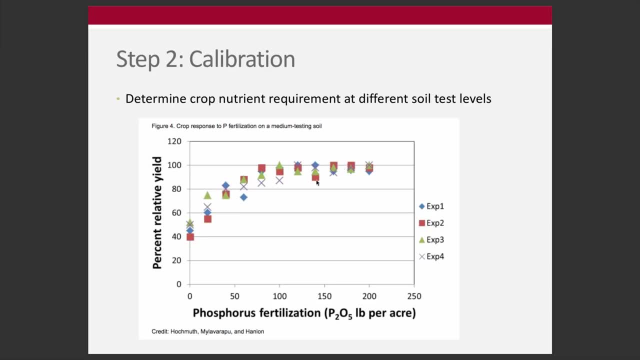 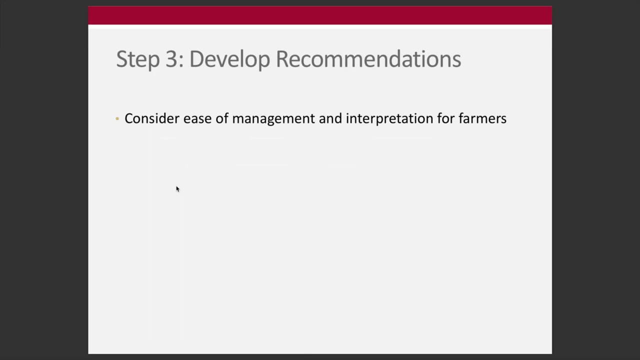 There's no additional response. that happens, But if we only apply 20 or 30, we can still see some increased yield. We're going to talk about this relative yield here in a second. So then the final step is developing that recommendation. 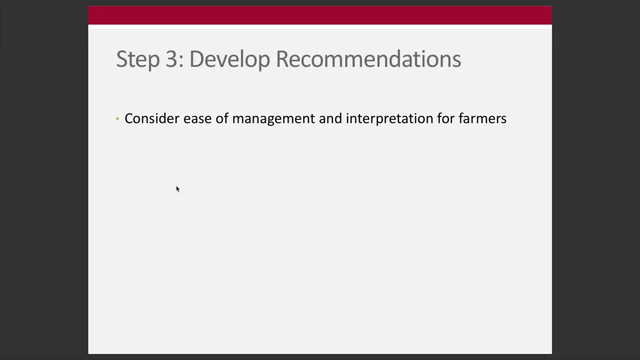 And this is kind of where we have to bring in a number of things like just a practical view of how easy it is going to be to manage this information. how will the farmers interpret it? how will they actually use that information? So recommendations are often not perfectly scientific. 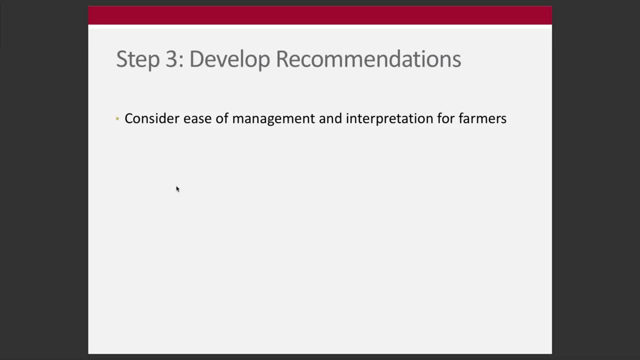 That is, they're often not exact, But you know there's an element of just kind of ease that are built in. So again there's these tradeoffs between how much you know, how practical can it be for a farmer? 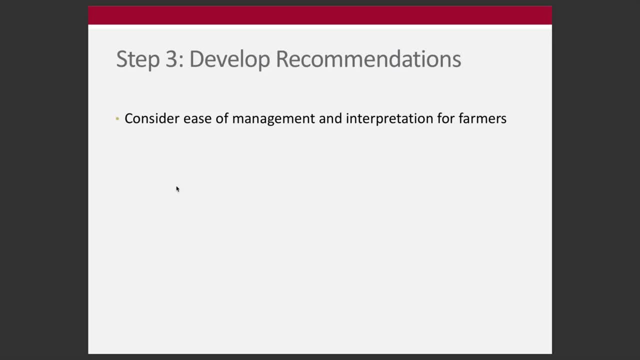 versus. are we going to provide recommendations Like I mean? you know, an easy example is like providing recommendations based in saying you should apply 62.45 pounds of phosphorus per acre, for example. Well, 0.45 of a pound on an acre basis is. 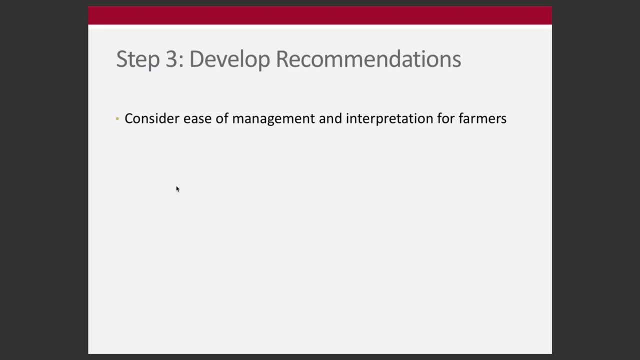 a farmer is never going to be able to measure that right. And so because our applicators, our fertilizer applicators, aren't that precise. So you know, maybe instead of 60,- whatever the number- I just said 62 something. 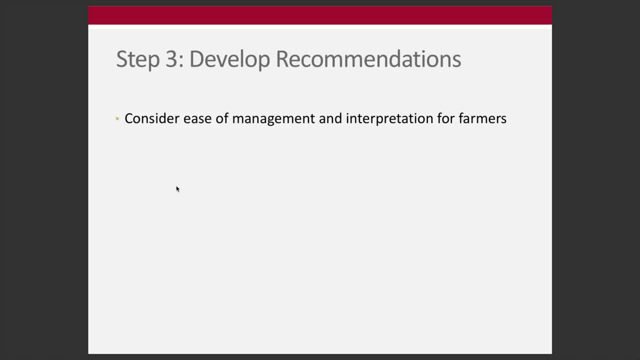 maybe you're just going to round it up to 65 and make it a nice even number, or maybe down to 60 and make it an even number. So again, this is where this kind of human interpretation comes in and just helps make that recommendation. 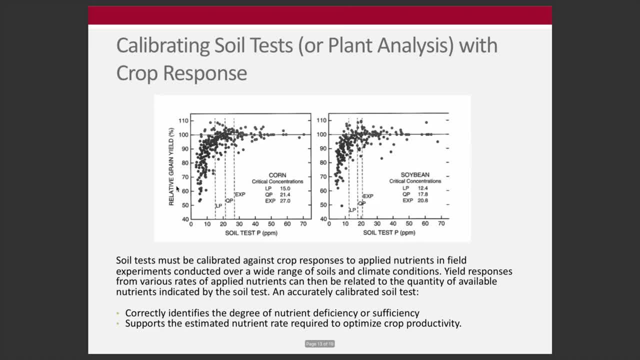 easy to remember, easy to implement for a grower, Okay. so calibrating soil tests with plant response or crop response, Again showing similar things. This is data from Iowa, Antonio Mallarino, out of Iowa State. Here's soil test P. 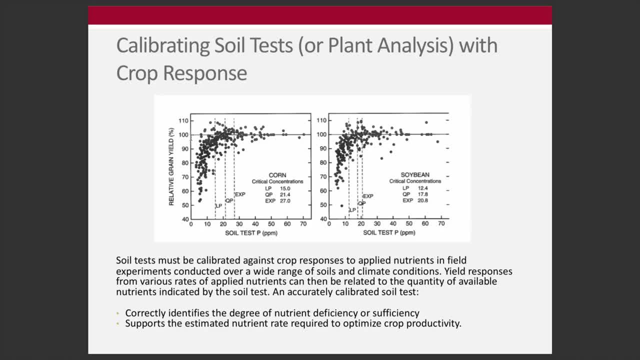 This is corn and soybean, And then here's relative grain yield. So any value less than 100 means that we're actually losing yield when we're at 100, or you know? Here is, ladies and gentlemen, here is the dark reality of soil fertility. 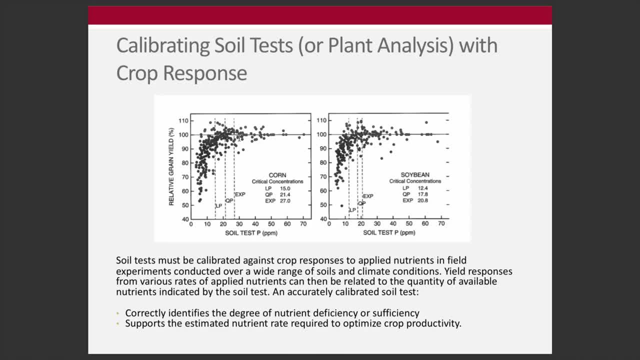 And it's that it's really messy, right, And you know, you look at this and I ask, I'll ask you, where does this actually break where we can actually say you should apply fertilizer or you don't have to? Well, of course, it's not very clear cut. 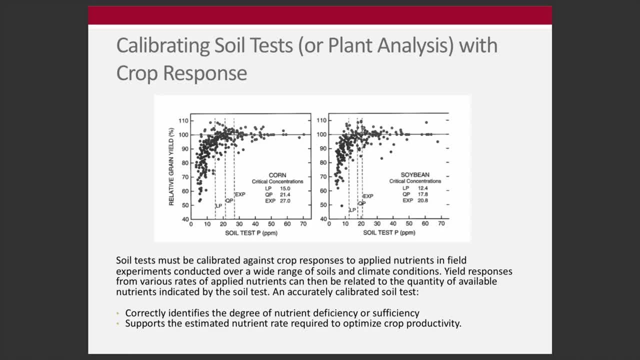 exactly where that point is. And so, again, this is this kind of element of when you're developing a recommendation, trying to be conservative, So you want to ensure that a grower or whoever might you know, not be under applying, but we don't want to be super conservative. 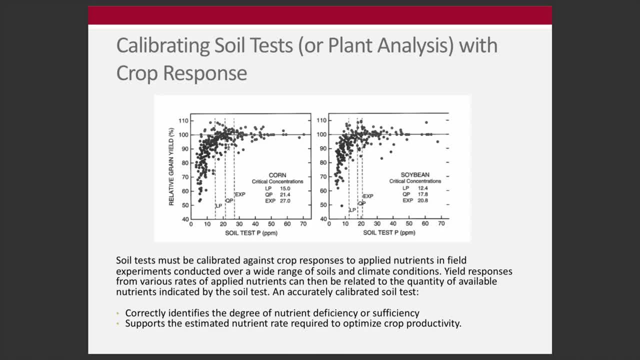 And so everyone's going to consistently be applying more than they need LP, QP and XP. So these are three different types of curves that we fit- a linear plateau, a quadratic plateau or an exponential curve- And depending on that curve, we can get these idea. 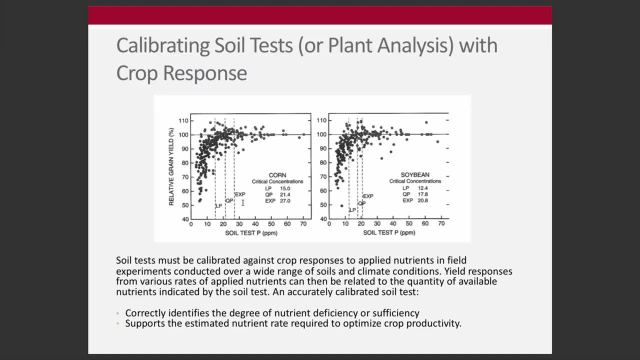 of different critical levels. Okay, so this is a new term And we'll talk a little bit more about this later. But this idea of a critical level being this magic, this magic soil- test value of when you should apply or you shouldn't apply, 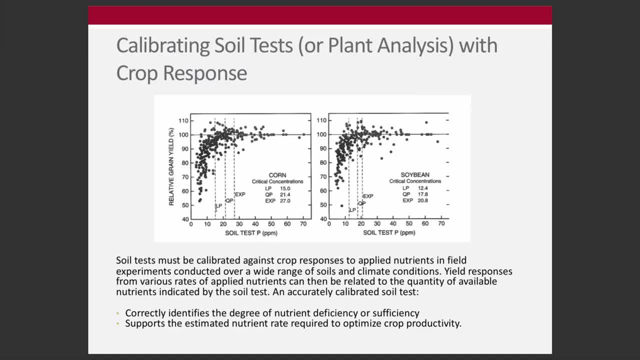 Or you know whether you're going to likely see a crop response to fertilizer or where you're not. Okay. so we can see in this data set, at least for corn, the LP, the QP and the XP, the linear and quadratic plateau and the exponential. 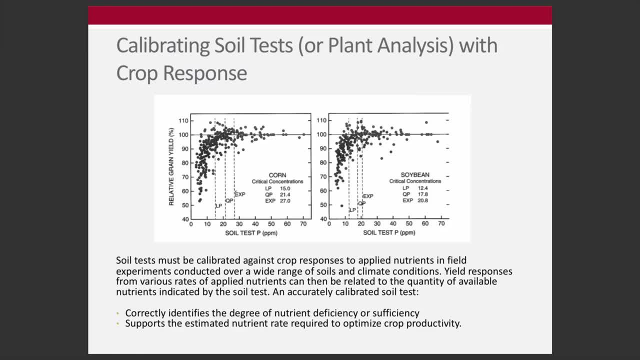 produce different, very different critical levels right. So 15,, 21, and 27, almost a two-fold range here. Now we can look at the response or the fit of that curve and make inferences based on which one's better. 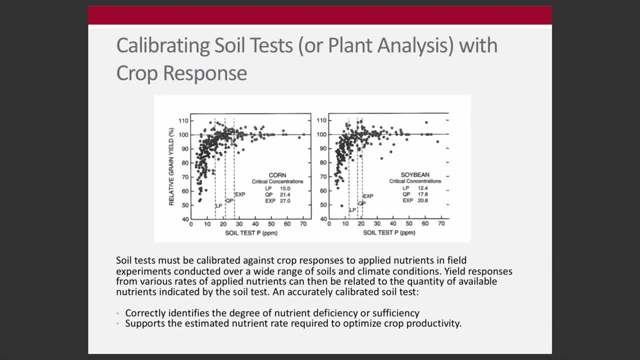 But the reality is that you know this is very common to find in soil fertility, And so there's some kind of fudging or just best guessing, And we need to recognize that when we find a soil test value and say our critical level is 15 or it's 20 or it's 30,. 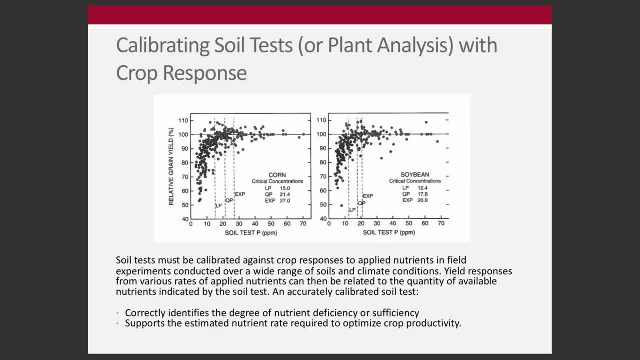 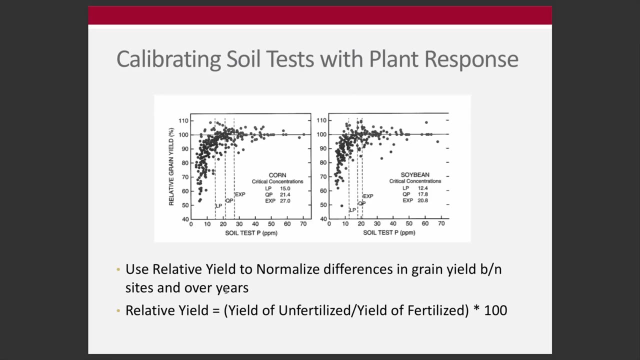 it's not a magic number that's going to be perfectly consistent every single time. okay, This idea of relative yield: we use this to normalize differences in grain from year to year, or whatever yield from year to year, So this doesn't have to apply, of course, to field crops. 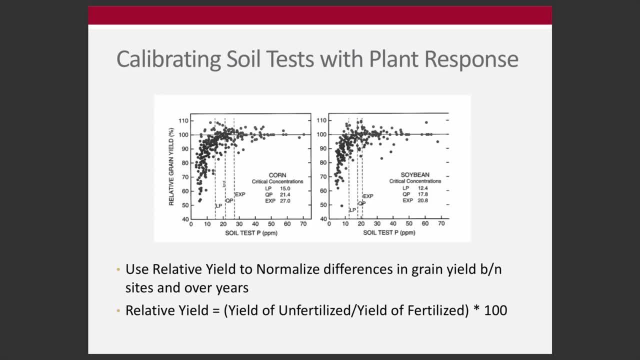 But year is going to be, it's going to drive yields regardless of the crop. Some years are good, some years are bad, And so this calculation of relative grain yield on this axis is the yield of the unfertilized divided by the fertilized times 100. 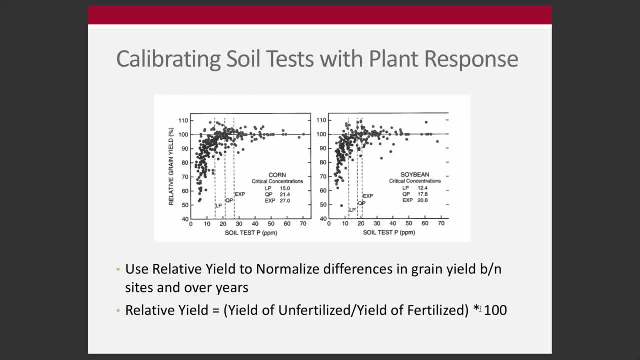 So that's pretty simple. So that essentially normalizes everything, puts it on 100% scale. If it's less than 100, we're seeing yield loss. It can actually, as you can see, be greater than 100.. These points up here show that fertilization actually 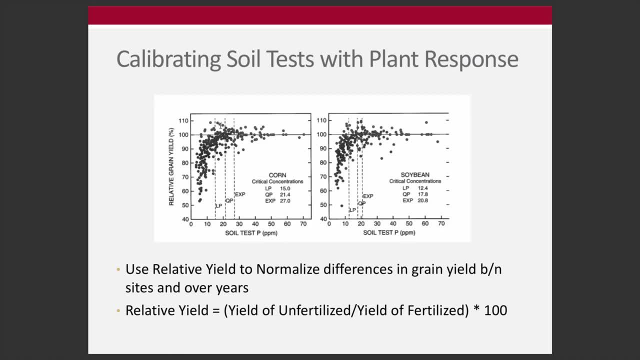 if the plots that were not fertilized yielded more than the plots that were fertilized And we infer then that that's kind of random noise, It means that the plots were not fertilized or limited, Whatever that nutrient we're applying. Okay, so again these kind of basic shapes. 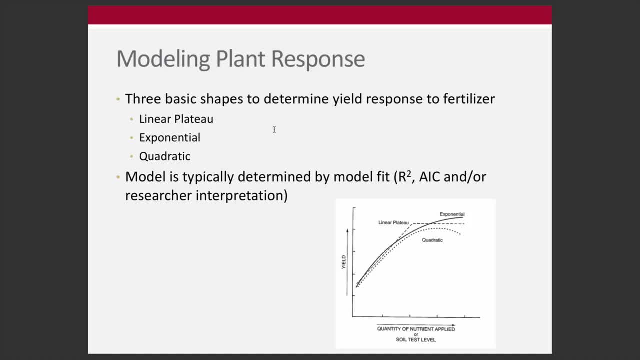 to determine yield response. So there's a linear plateau, an exponential, a quadratic, sometimes a quadratic plateau, And we will use R-squareds or AICs or just looking at the data, kind of a subjective interpretation of that, to kind of determine the best model fit. 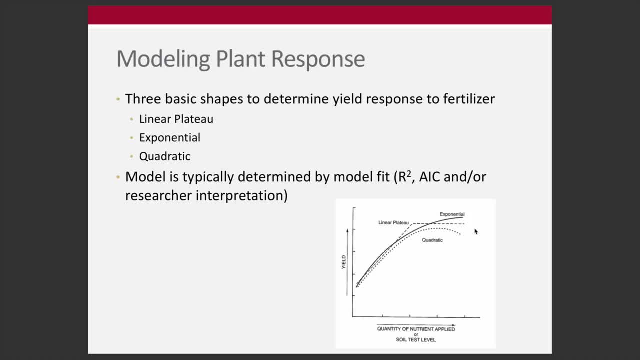 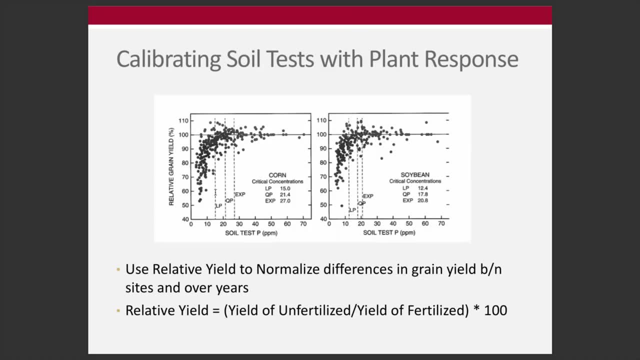 So these are kind of typically how this is done, And it's why we often get this very talk about this a number of times. this generalized relationship of yield loss or productivity declines at low, say, soil testing level or plant nutrient concentration. 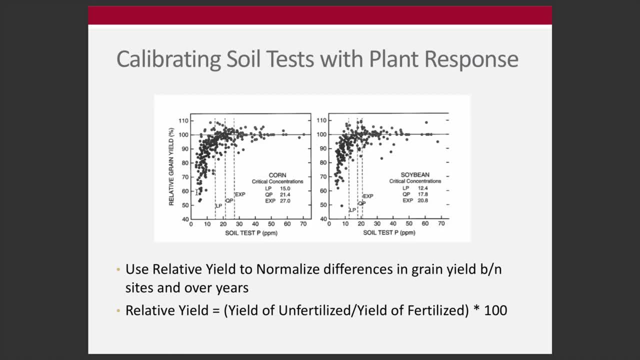 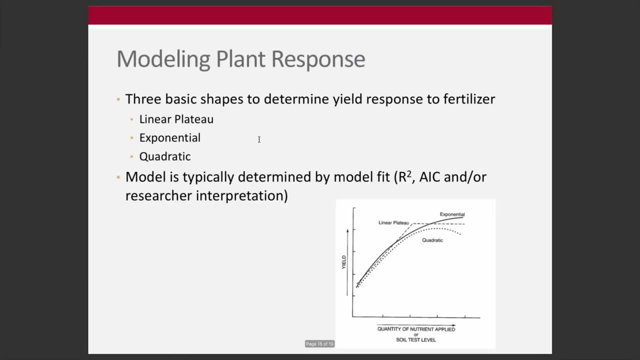 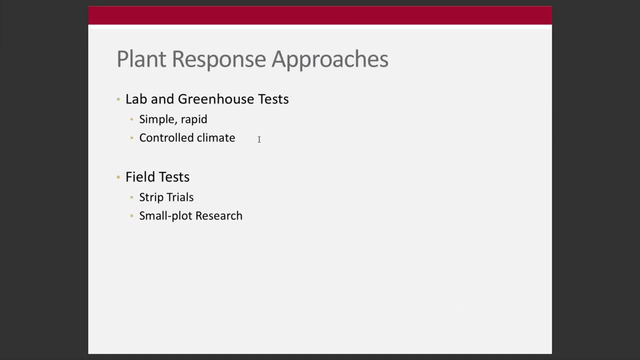 And as that increases, those start to plateau and become non-significant over time. Okay, So developing plant responses: We can do this in the lab or the greenhouse. These are simple, rapid, controlled environments, But more commonly we want to do these in the field. 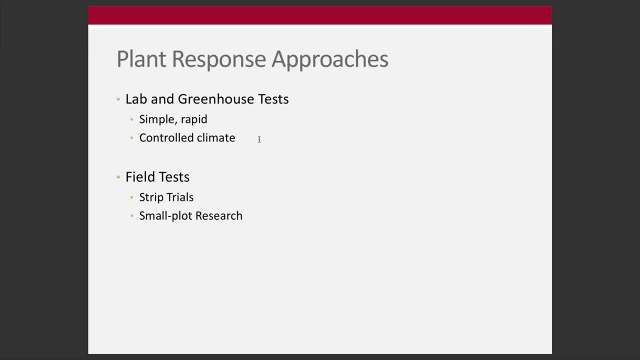 to make them much more realistic. You know, greenhouse experiments are often really difficult to extrapolate to the real world. okay, And so for field trials, we can think of either large strip trials or small plot research trials. So greenhouse trials where we might. this is. 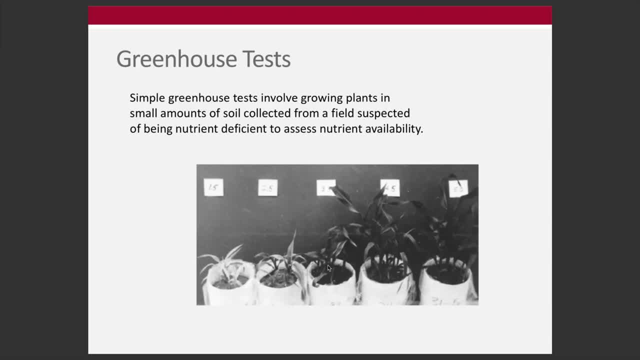 I can assure you this picture is from how long ago. but you know, whatever the nutrient we're applying at one and a half, two and a half all the way to five, and you can see it's clearly the soil and this plant. 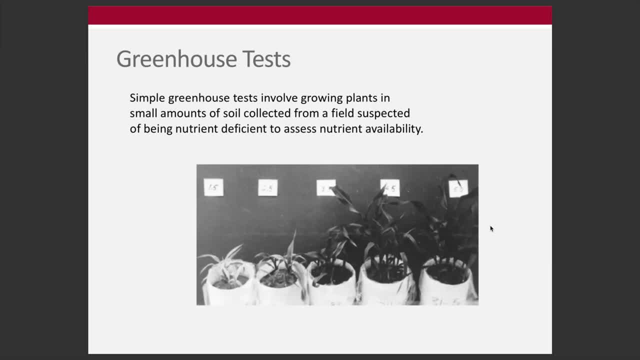 is responding to whatever that nutrient might be right. So we can do this and get some idea of levels, But again, because of these patterns, these pot experiments- unless the crop that you're growing is a potted plant, you know if it's. 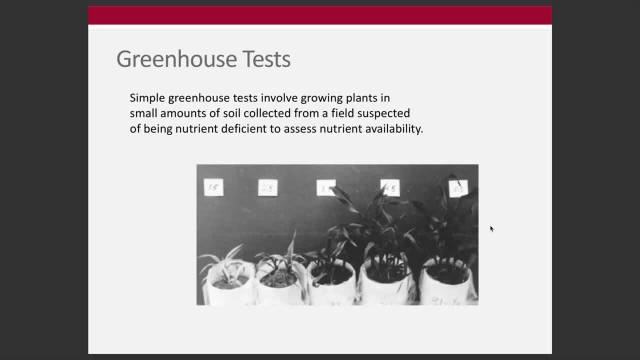 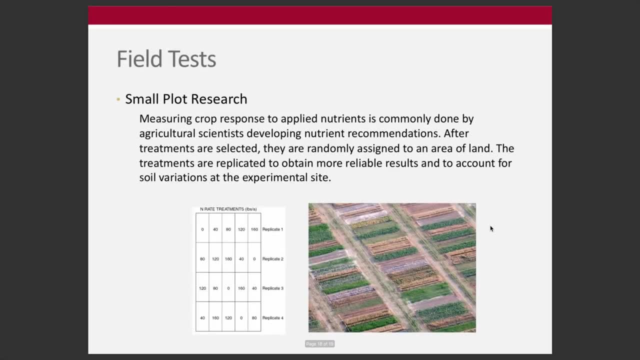 then this makes perfect sense. But if it's not, if you're growing in the field, then you're going to often get very different results. So small plot research: University scientists like to do this, but farmers often balk at this because they do not like. 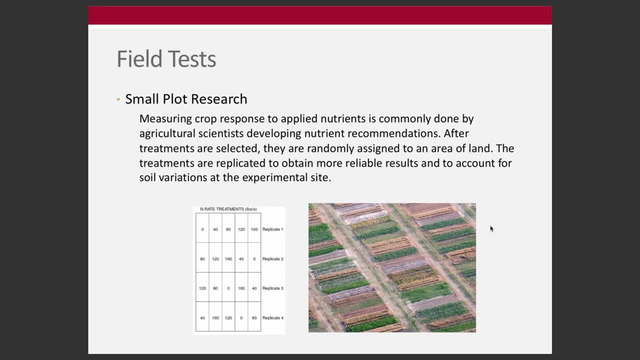 well, there's a number of reasons, but as university scientists, we typically like these because it controls the amount of variability that we encounter in any given field. It allows us to do multiple treatments Instead of just maybe one, two or three treatments. 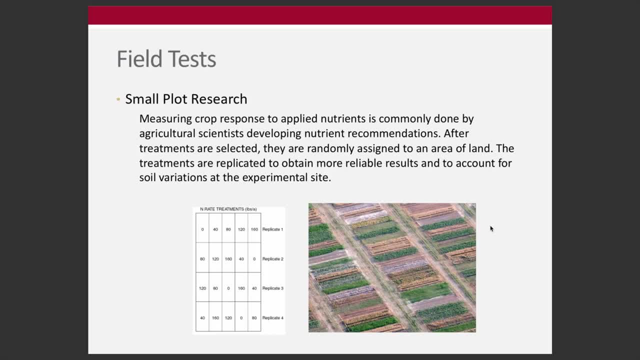 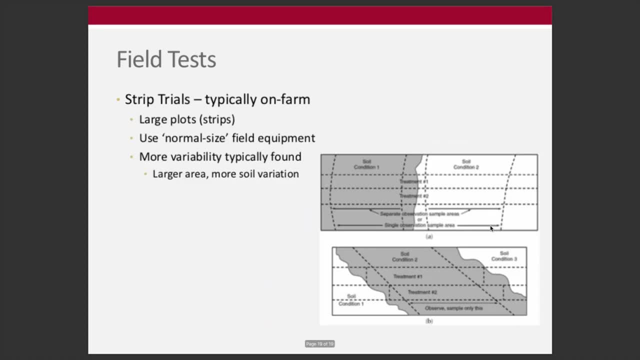 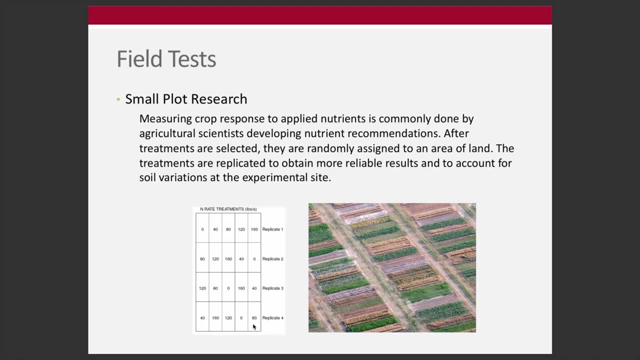 we can do, say, ten different treatments and get a lot more information. We will do this typically with a randomized complete block design, have different treatments and different replicates or blocks that we'll call Growers. you know we take the approach that we like both pieces of information. 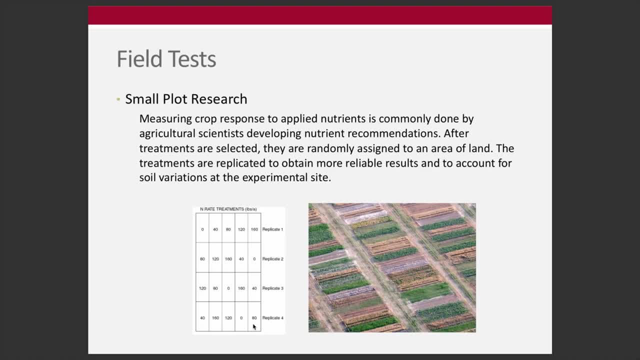 but farmers are often much more likely to believe research that comes from large strip troughs and especially comes either from their farm or from a neighbor's farm, or from a farm you know in their county, someplace close or local, instead of you know some faraway place in Worcester. 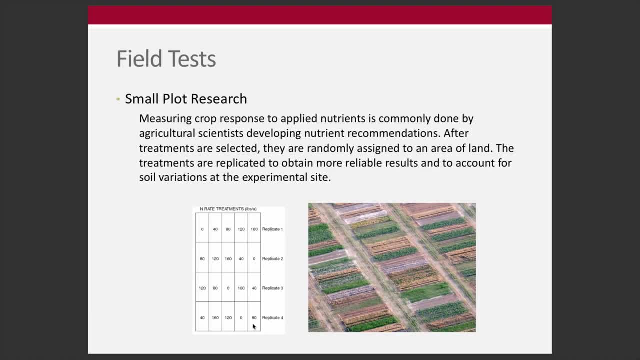 or whatever that you know, trials were ran, So anyways, there's a whole social dimension to that that we could get into. But you know, suffice it to say that there's a lot of small plot research that happens at university farms. 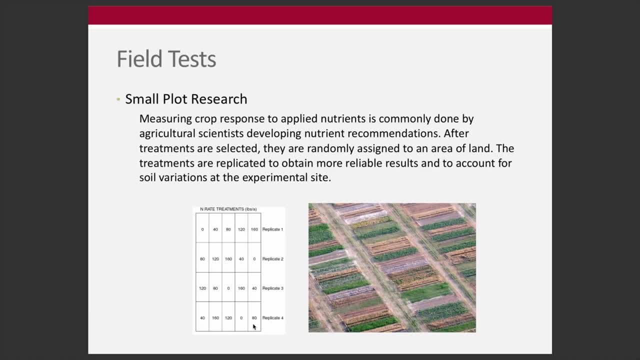 And we can take this. If we've got equipment- and we do this all the time- we can take equipment and actually implement small plots on a grower's farm right. There's no problem with that. It's just that we need typically specialized equipment. 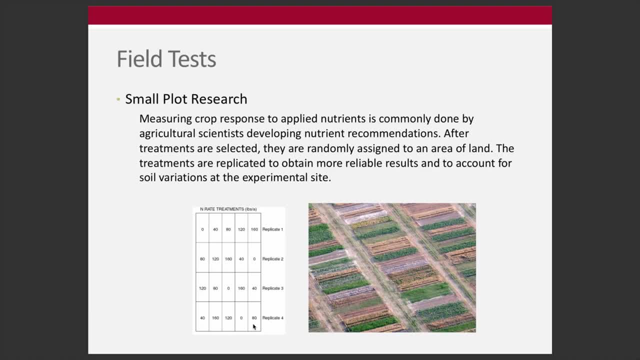 that are, you know, small planters, small combines, et cetera, et cetera. But this is commonly done, So the lines can get blurred, okay. And then, finally, is this idea of large strip trials, where you know we're using quote unquote. 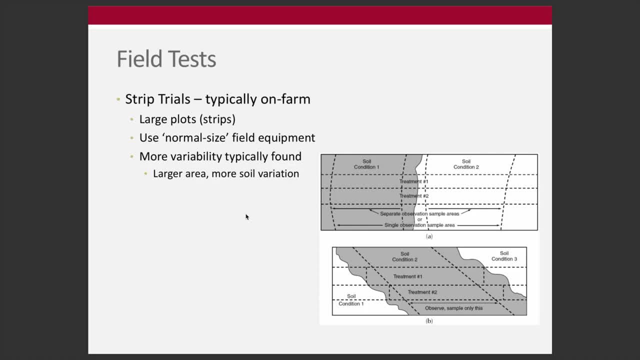 normal size field equipment and doing a small number of treatment, op like treatment, one like versus control. Phosphorus-fertilized strip versus, you know, a non-fertilized strip Or what have you. The problem with this is that these are typically much larger. 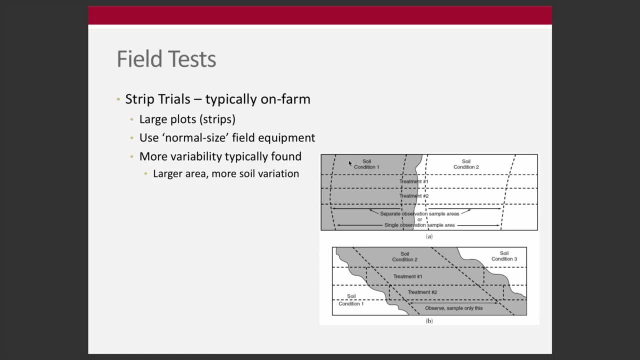 And as our field site, our actual field experiment, the area of that increases. Just, you know, from a probability perspective we're going to increase field variability. okay, So as field area, as the area increases, the variability is going to increase as well. 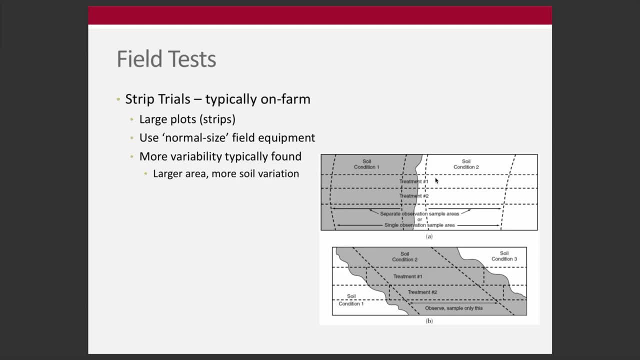 Very commonly, And there's very few instances, that's not true. So here you know, we've got two different treatments and then two different soil conditions, or maybe three different soil conditions, And this can really introduce a lot of noise, a lot of variability. 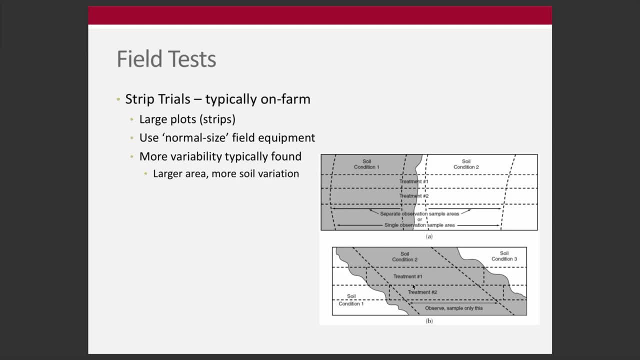 And it might really compromise the experiment. This is why a lot of people don't like to do this, okay, So anyways, just some tradeoffs. There's always tradeoffs in life, And here's one tradeoff between small plots which give you greater control.